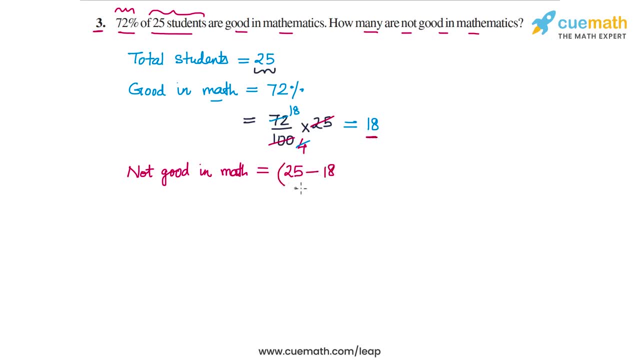 good in mathematics, which is 18, which we have calculated here. So 25 minus 18 is equal to 7.. So the number of students not good in mathematics is 7.. The other way to have solved the same problem is that, instead of calculating the absolute number of students who are good, 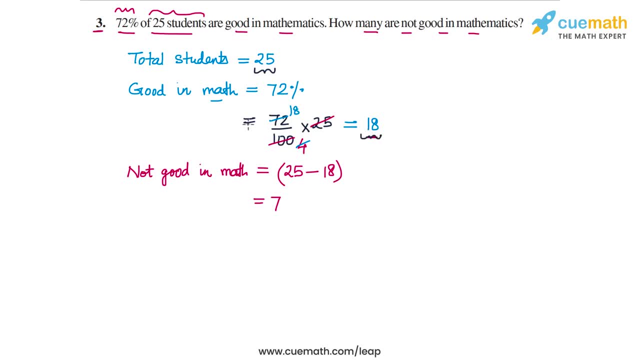 in mathematics, we can first find the percentage of students who are not good in mathematics. How can we do that? So we know that the percentage of students good in mathematics is 72%. This means that the percentage of students not good in mathematics, the percentage of such, 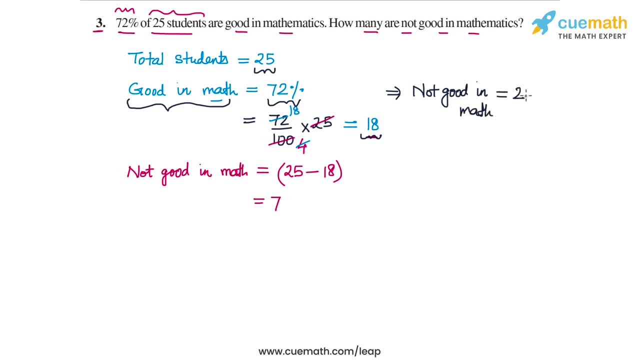 students is 100% minus 72% or 28%. So the percentage of students not good in mathematics is 28%. We can convert 28% into an absolute number, So that will be 28 by 100 into 25, which is: 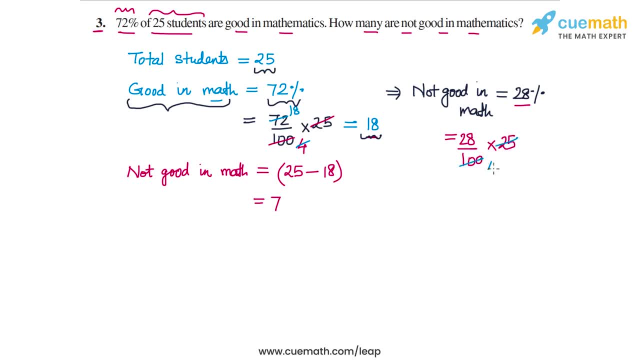 the total number of students. So 100 by 25 is 4.. And then 28 by 4 is 7.. So the number of students not good in mathematics is 7, which is the same answer as what we obtained in the first approach. So let me summarize the two approaches. We are told that the total 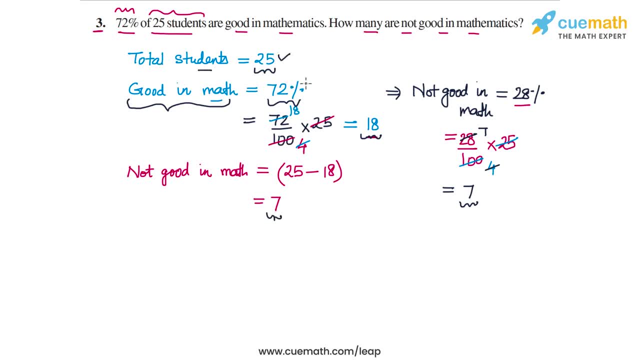 number of students is 25.. And the percentage of students good in mathematics is 72%. So in the first approach we calculate the number of good students, number of students who are good in mathematics, which is 18, and then subtract that from 25 to get the number of students not good in mathematics. 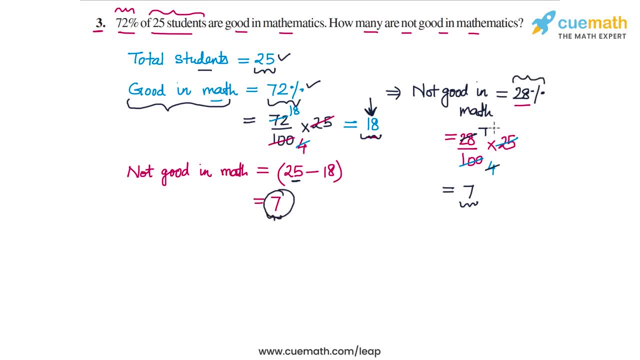 In the second approach, we find the percentage of students not good in mathematics, which is 100% minus 72% or 28%, And then we convert this into an absolute number: 28% of 25, which is 7.. So both approaches give us the same answer, which is that seven students are not good. 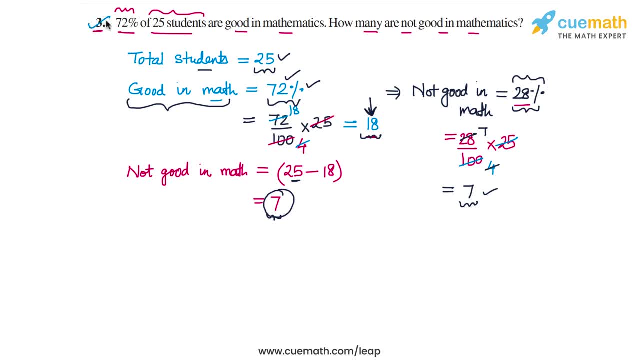 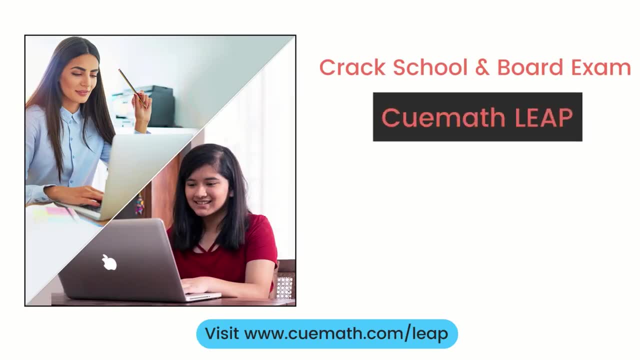 in mathematics. With that, question three is completed.